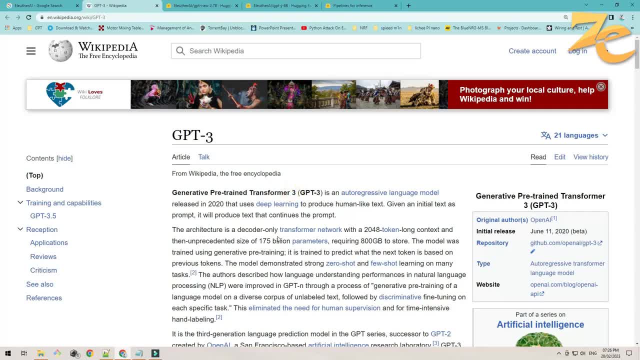 So basically GPT-3 is developed by the OpenAI company name. And they have some their own models. Basically they are highly trend data set models. So all their value lies in that model. But the GPT's some architectures are there like GPT-3 that are open source. 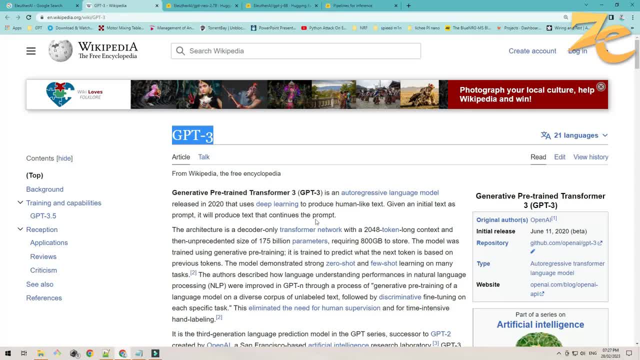 We can use that architecture. And also, there are some pre-trend models openly available. 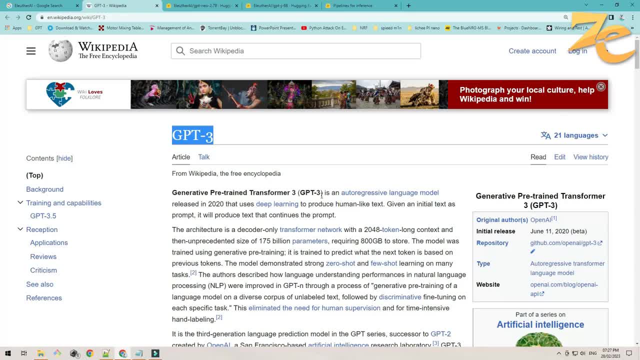 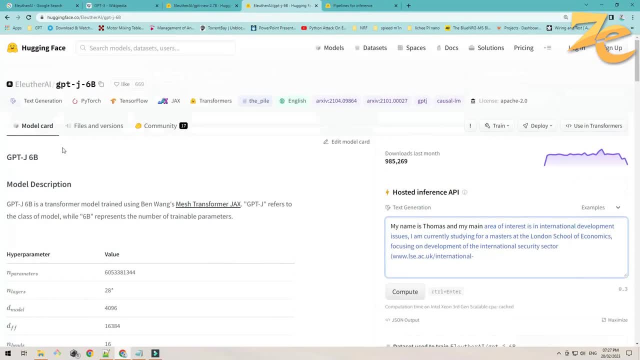 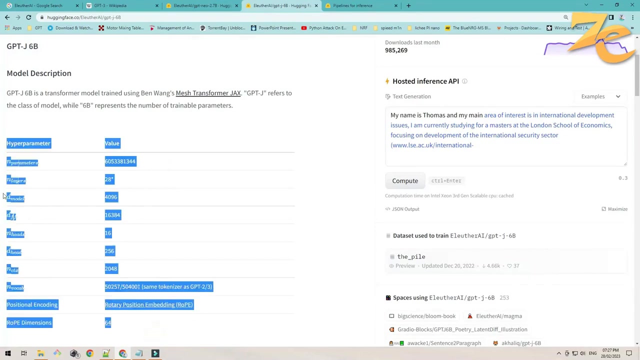 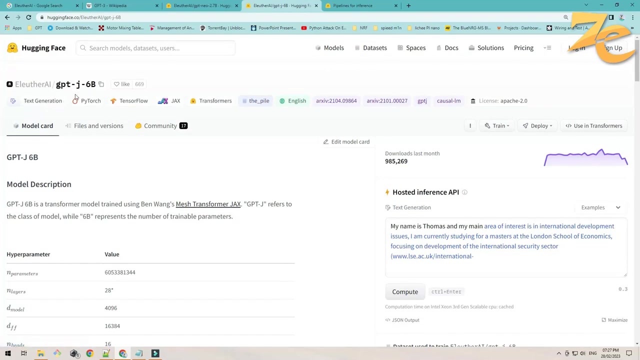 So what are that models which is equivalent or better than the GPT-3? So first model is this GPT-J 6B. So here 6B means this model is trained on 6 billion parameters. You can see the rest of the parameters. Rest of the configuration of this model. So basically it is as per the testers of this model. 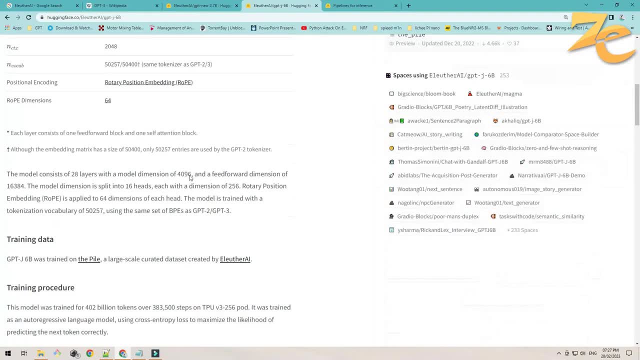 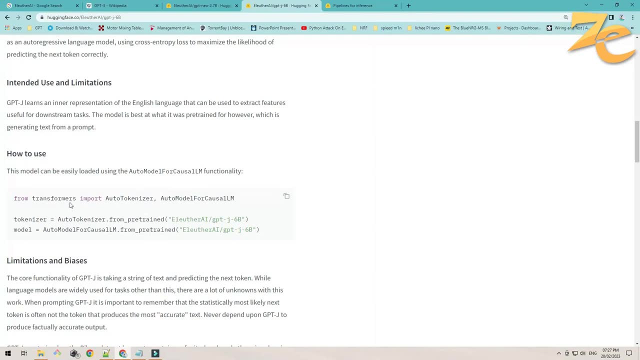 They said that this model is better than GPT-3. So we have this model we can download and use the transformers to load the model and generate the predictive text. 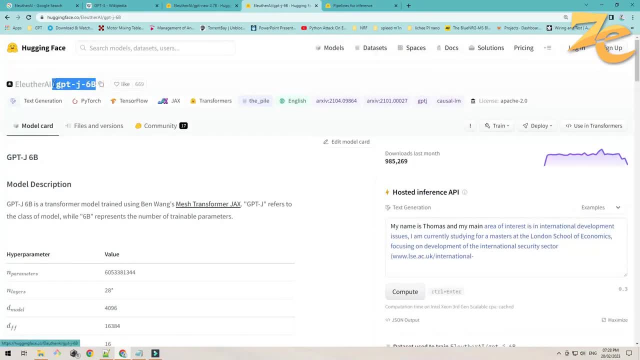 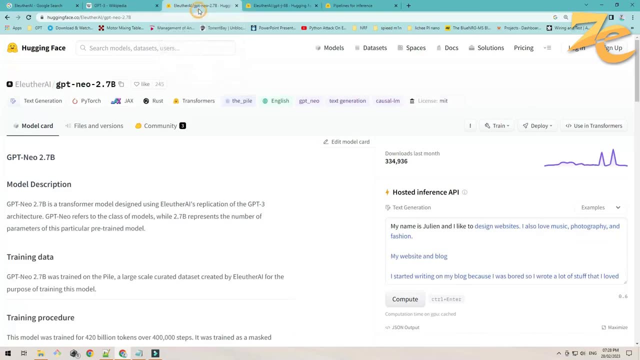 We will not use this model in this video. Because it required high configuration device. We have less power of GPU here. So the alternative is GPT-NEO 2.7B. Basically this model is trained on 2.7 billion data sets. Also this model also required too much power. So the alternative is their 1.7B. 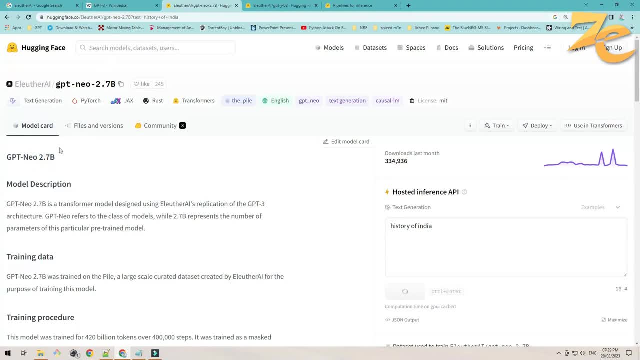 This is their 1.3 billion parameter trend model. That is nothing but the GPT-NEO 1.3 billion. 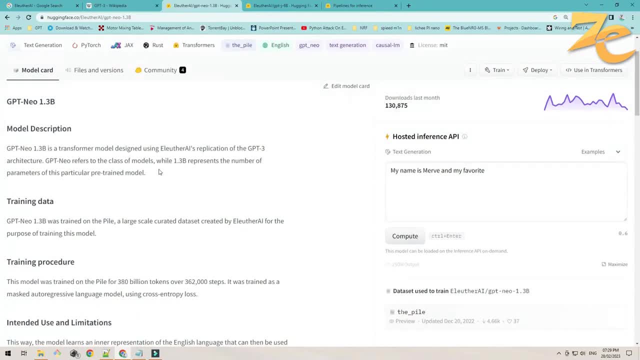 So this model. We will going to use this model. This is also sufficient for the basic predictive text generation. 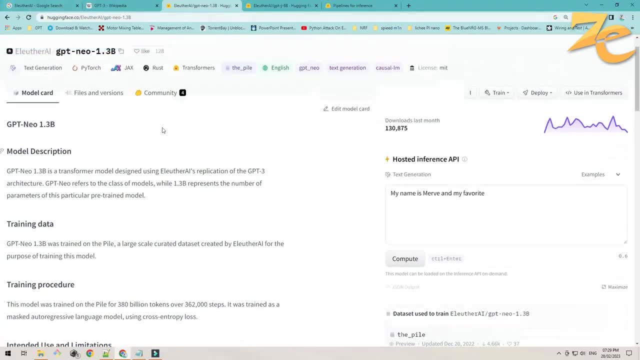 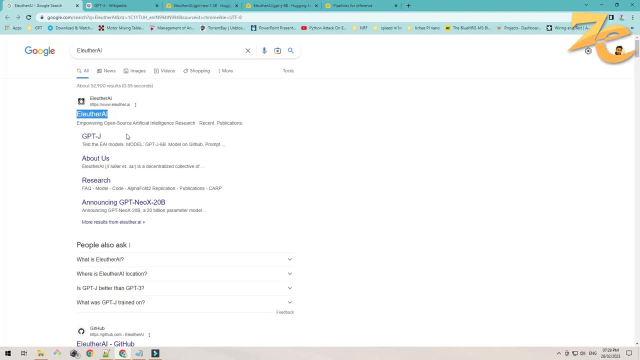 Who created this model? So basically Eleuther AI company. Means it is not a company. It is a community actually. 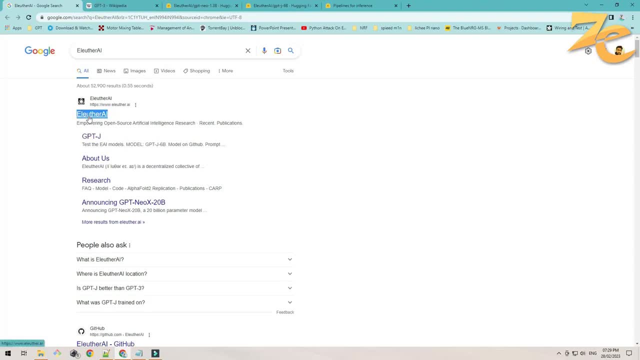 They make this GPT-NEO model. And also working on the future model like this. GPT-NEO X 20 billion. So this is equivalent to like train on 20 billion parameters. 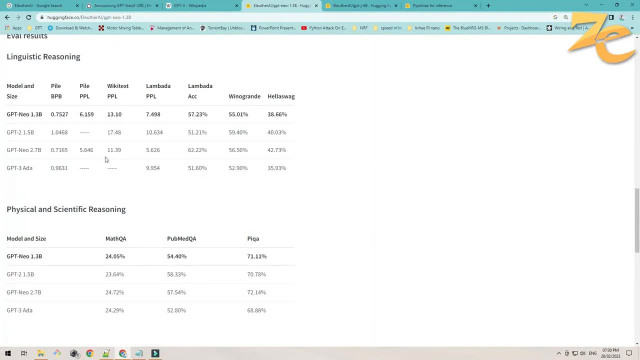 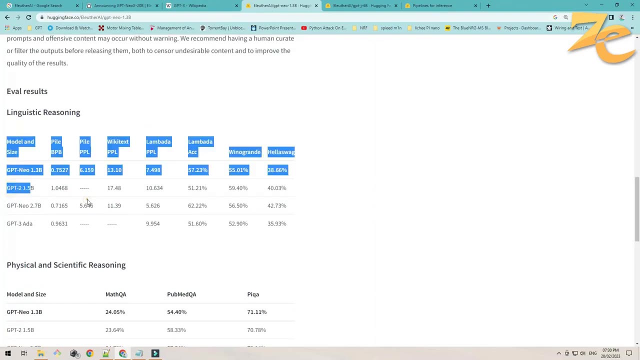 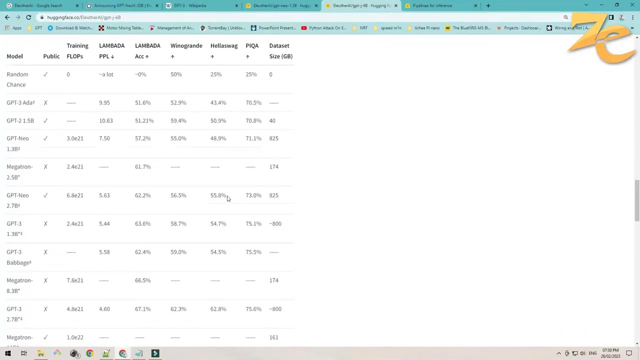 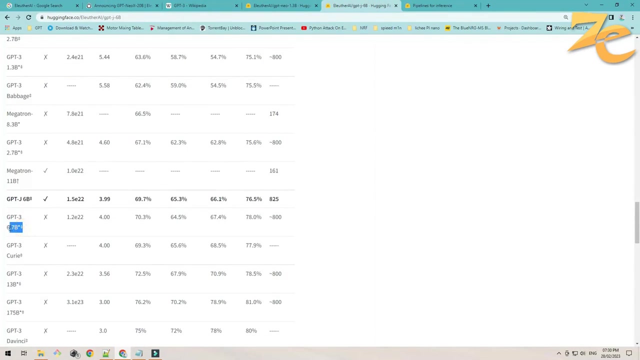 You can also see the comparison of this model. With the same models present. Here is the 6B model comparison. GPT-J6B model comparison with the GPT-3 also. So basically GPT-3 is trained on 6.7 billion parameters. 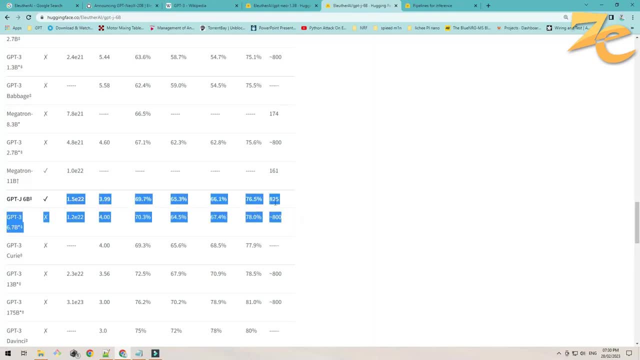 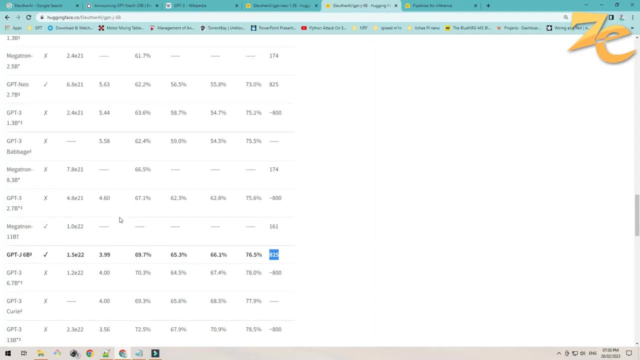 And if you see the score. You can see it is quite better than the GPT-3. 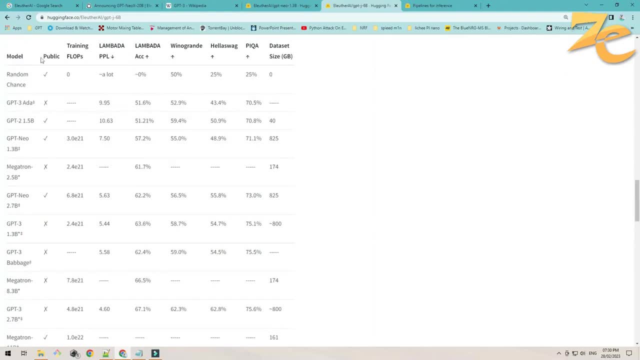 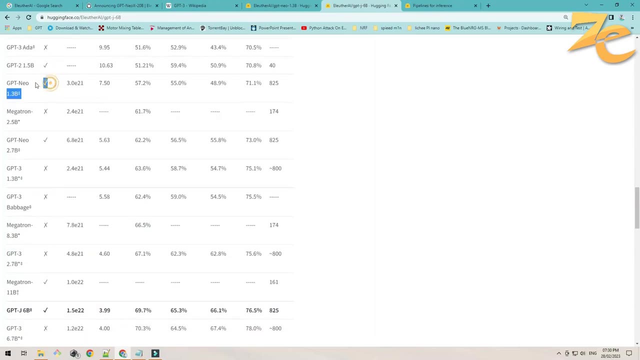 And also it is publicly available. So there are some other models too. Like GPT-2. It is also public model. GPT-NEO 1.3. So basically we are going to use this model. And also one. Famous model is this Megatron. Basically it is trained on 11 billion parameters. And the latest that is coming in market. Is nothing but the GPT-NEO X 20 billion. 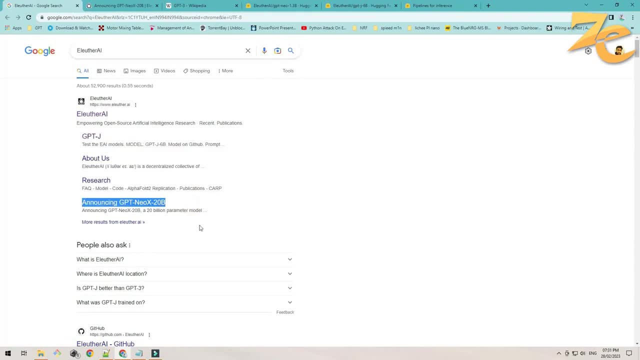 It is highly means trained on 20 billion parameters. Okay. 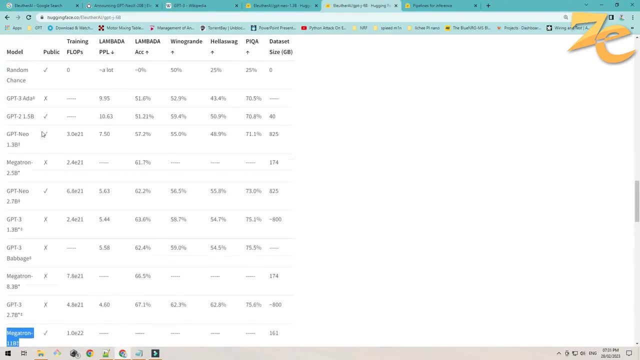 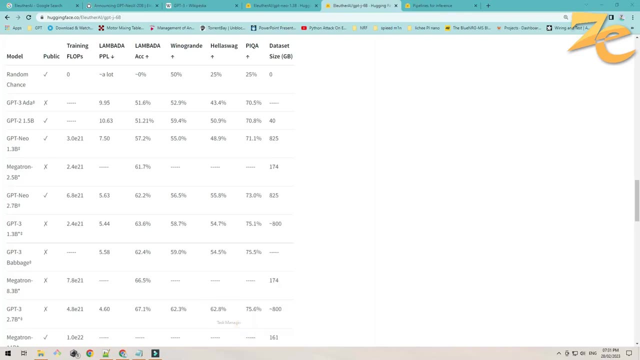 So let's see how we can use GPT-1.3 in Python. So let's see my PC configuration. So my PC having this GPU. 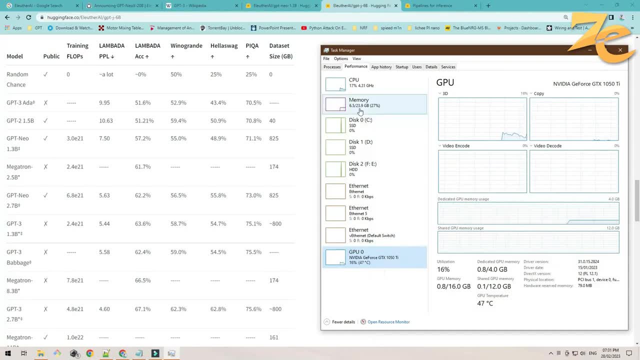 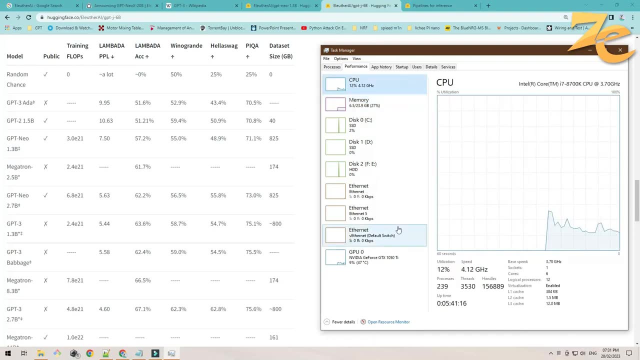 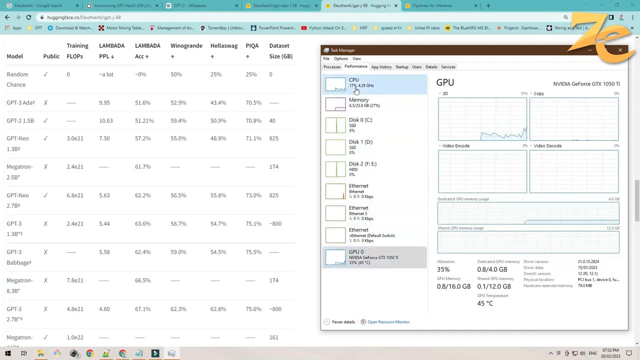 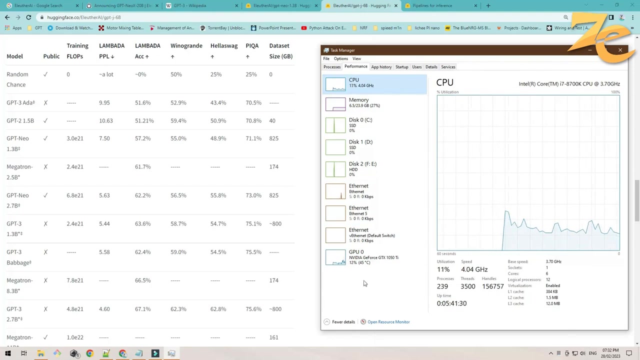 Nvidia G4X GTX 1050 Ti. And 24GB of RAM. CPU is Intel i7 8th generation. So basically we are not going to use GPU here. Because the model we are using. Is the float 16. That can only run on the CPU. 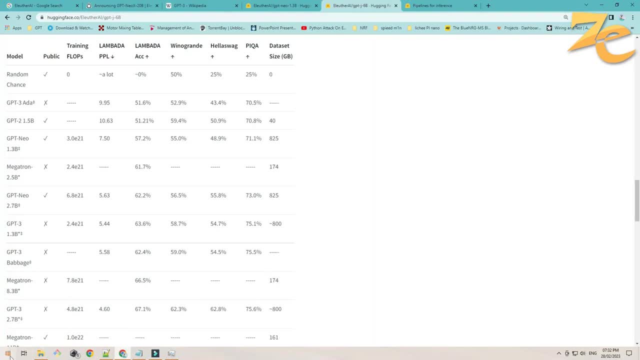 So let's start the coding. First you have to install. 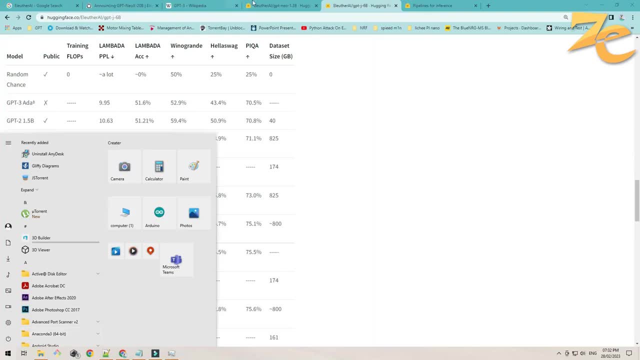 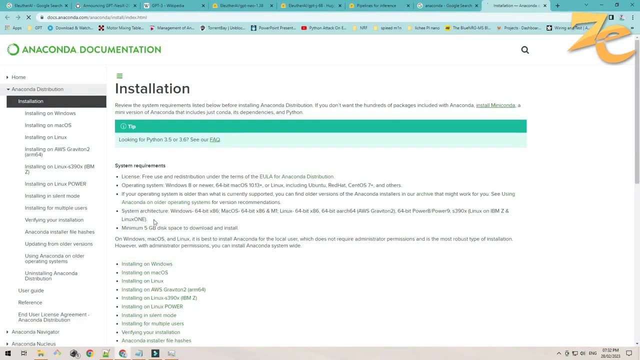 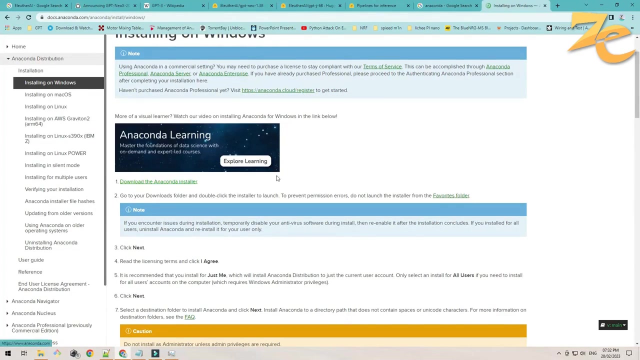 Anaconda. Basically you can go to. Anaconda. Or search on Google. You will find the installation link. Click on the Windows installation. Here download the Anaconda installer. And just straight away install it. You will get the console. 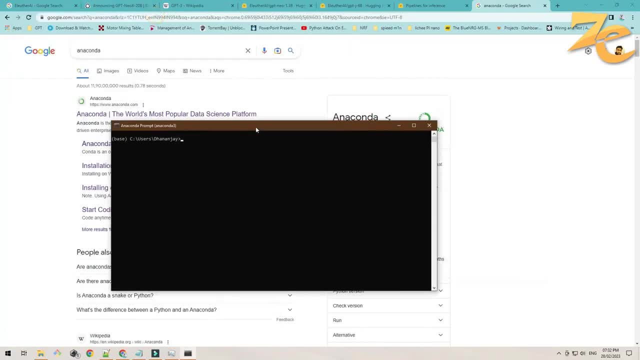 For Anaconda here. In this you have to create. Virtual environment. 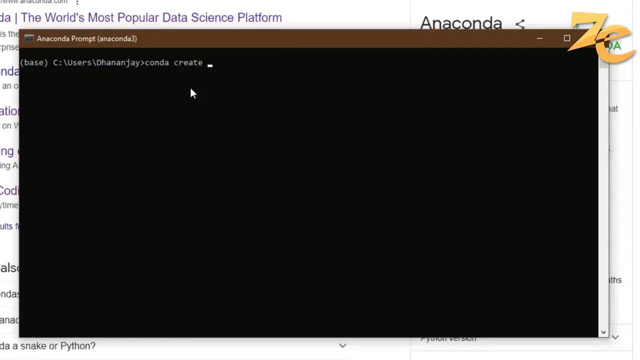 By giving the command. Anaconda create-n GPT. 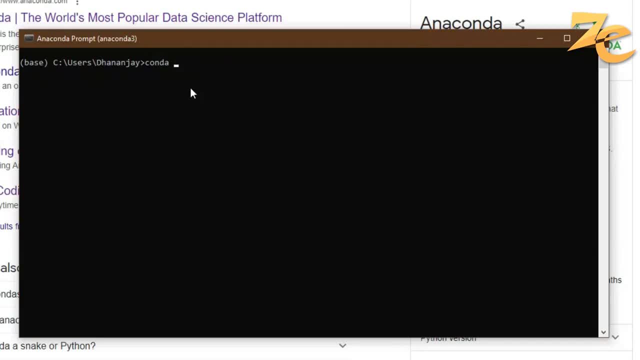 So I already have created. The environment. 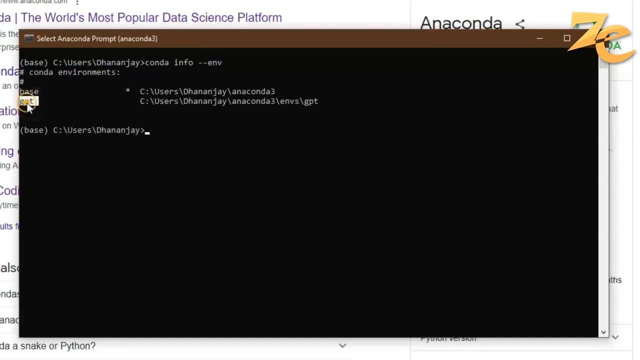 We will just simply activate. This environment. 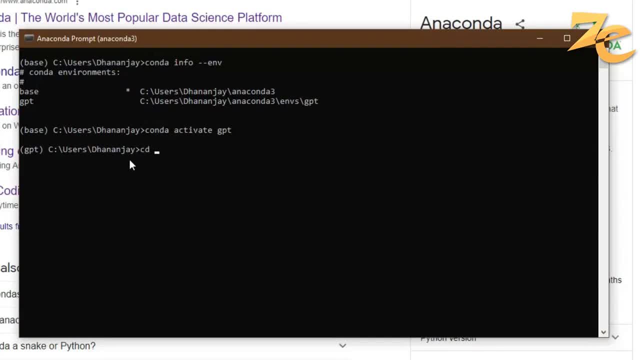 And navigate to. Our GPT data set. Here I have. 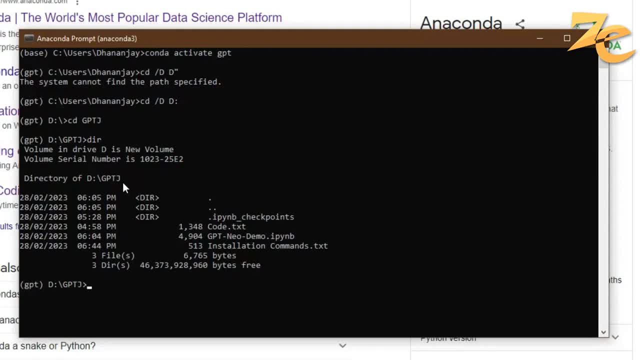 Tried to run the GPT-J model. But this. PC configuration is not sufficient. If you want to run the. GPT-J model. 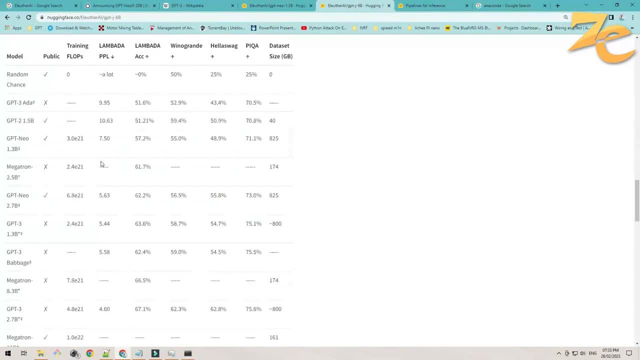 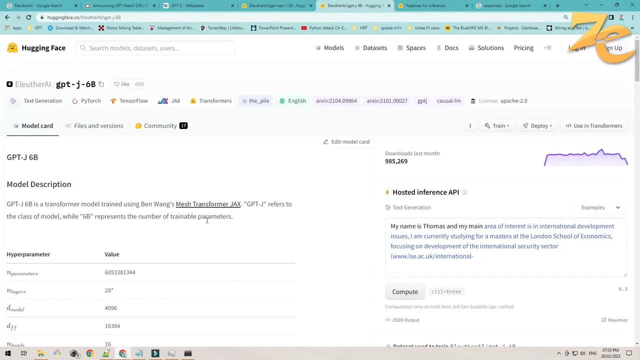 Which is 6B. So it requires. I guess. 12. 12 gigs of VRAM. Means. You need a. GPU. Which having the. Memory of 12 gigs. 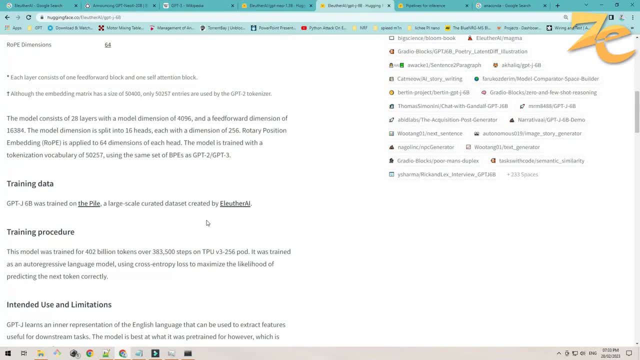 And that much. GPU is not available. At my. Local machine. So I. Go with the. Lower trend model. So. 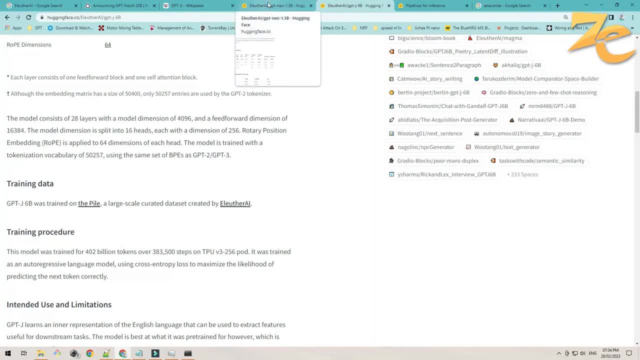 It requires. At least. You have 6. Or 4 gigs of. GPU. 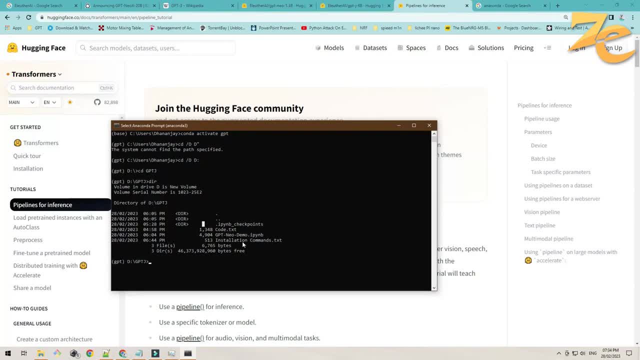 So. Just. First. Before. 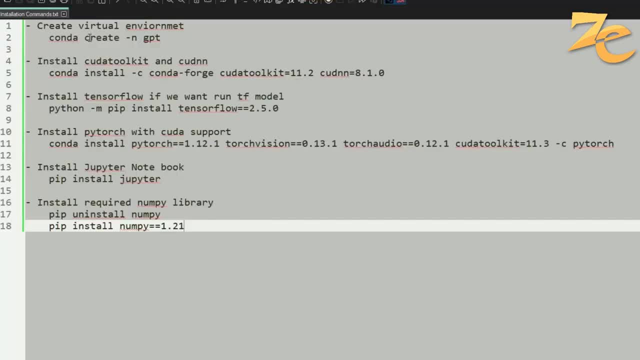 Opening the notebook. You have to. Give some command. Which is. This one is for. Creating environment. Which I. Already have. Installed and. 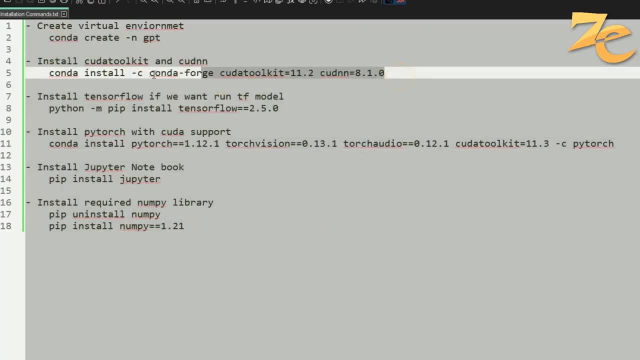 Set up this. Environment. So later. You have to install the. CUDA. CUDA toolkit is. 11.2. And. CUDNN. 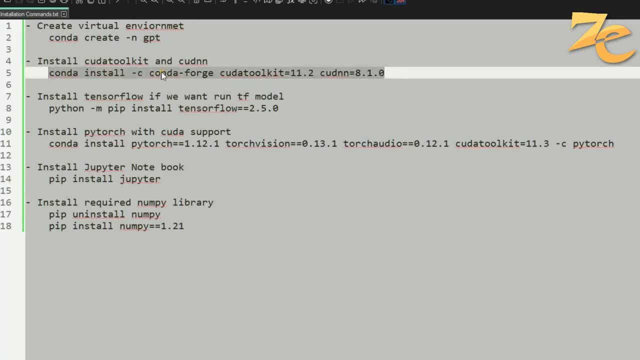 Is. 8.1.0. So. We are. Installing this from. Conda first channel. The next thing. We. We. 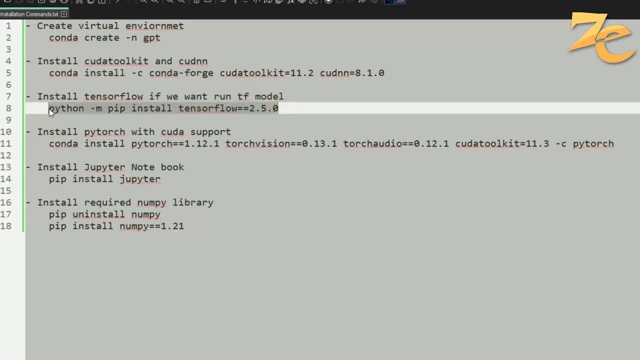 Have to install the. TensorFlow. 2.5. TensorFlow here is. Required. Because there are. Two type of. Models. Available. 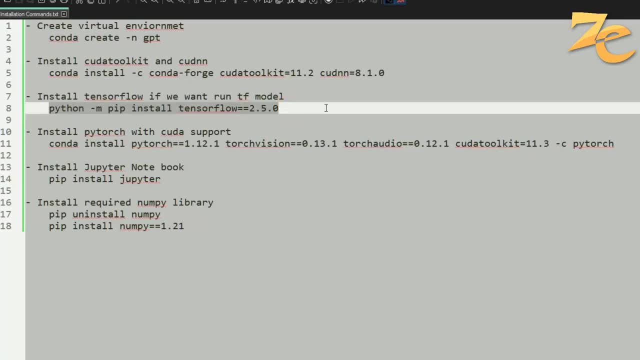 One is a. Torch. Model. And. Other is. A. TensorFlow. Models. If. 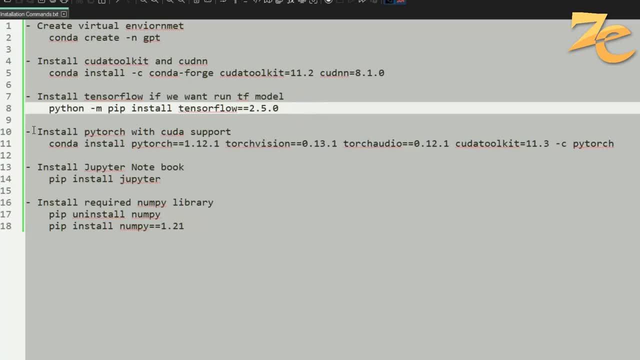 You. Want. To. Run. A. TensorFlow. Model. Then. You. 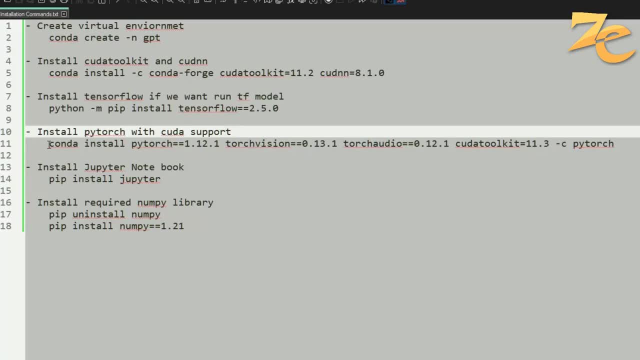 Can. You. Have. To. Install. This. TensorFlow. You. Need. 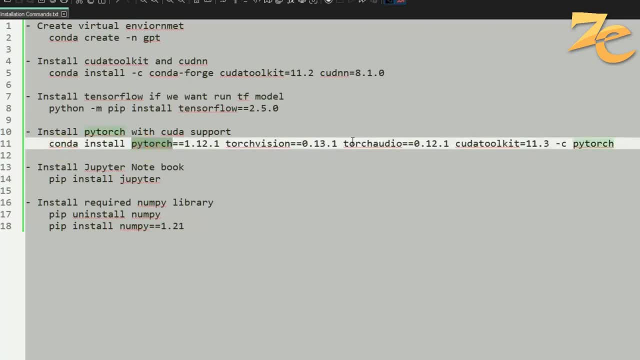 To. Tell. Conda. Implicitly. That. You. Want. The. Version. 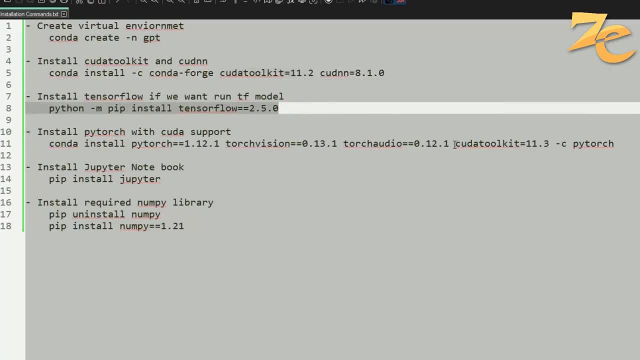 Of. PyTorch. Which. Is. Compiled. On. CUDA. 11.3. So. 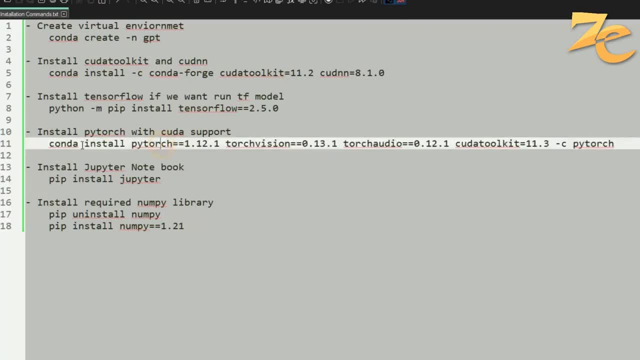 Here. We. Have. Installed. CUDA. 11.2. Which. Requires. For. 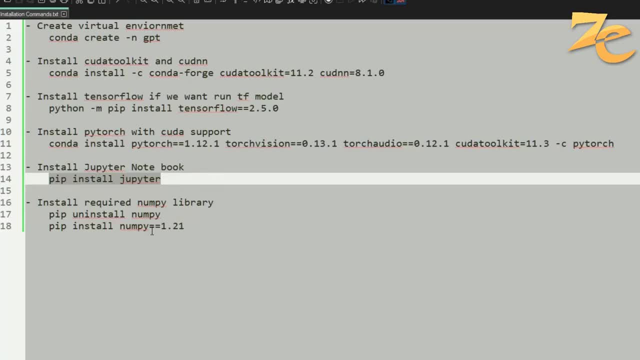 After. Installing. Jupiter. Notebook. I. See. That. The. NumPy. 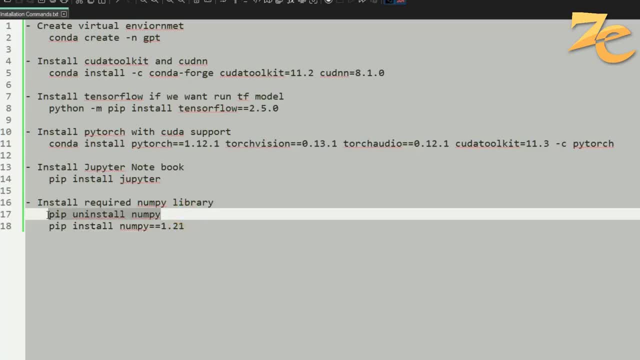 Version. Is. Get. Changed. So. The. NumPy. Version. We. 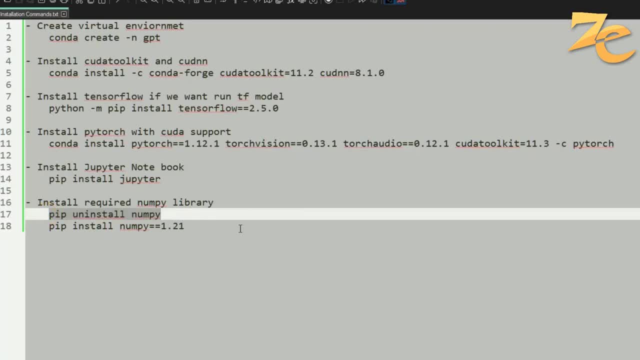 Required. Is. This. 1. 2. 1. So. We. Have. 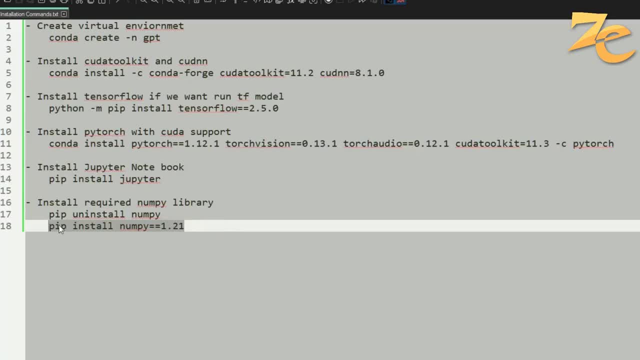 To. Uninstall. And. Then. You. Install. The. NumPy. With. 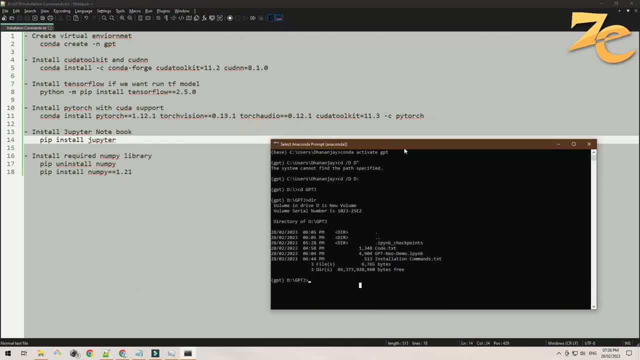 A. Specific. Version. 1. 2. 1. After. Setting. This. 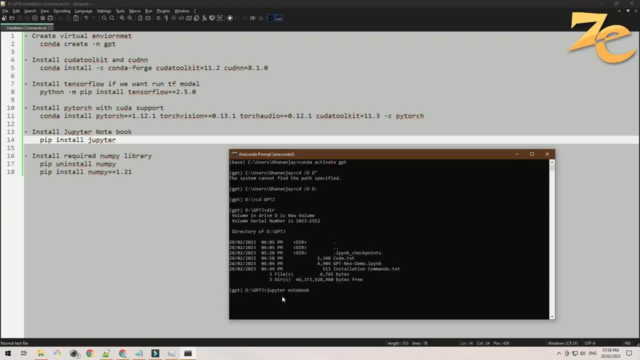 You. Will. Have. GPT. Environment. Okay. So. We. Just. Start. 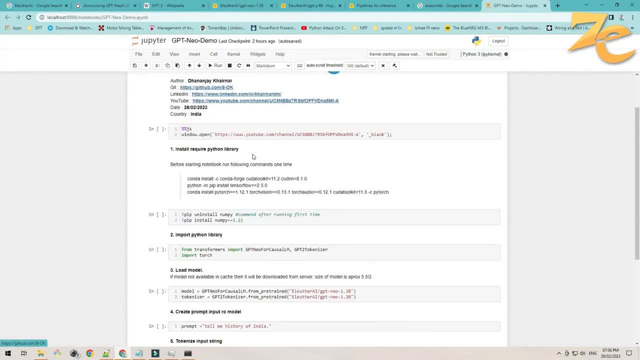 The. Jupiter. Notebook. So. Just. Start. Executing. This. 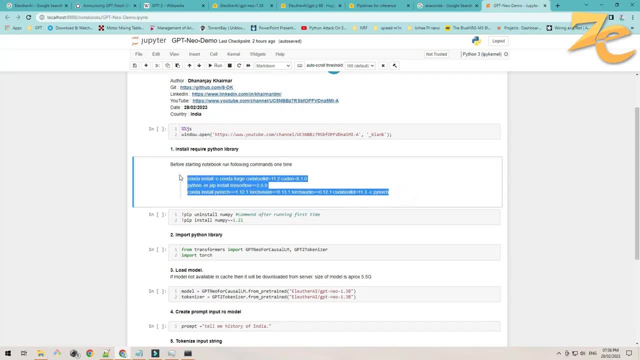 Here. Also. You. Have. To. Mention. That. Command. Which. 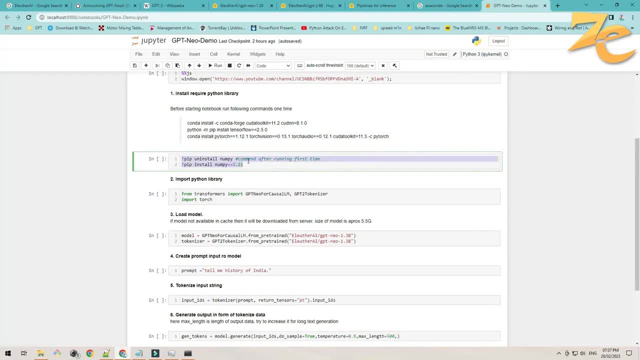 Already. I. Have. Given. You. Can. Run. This. Command. 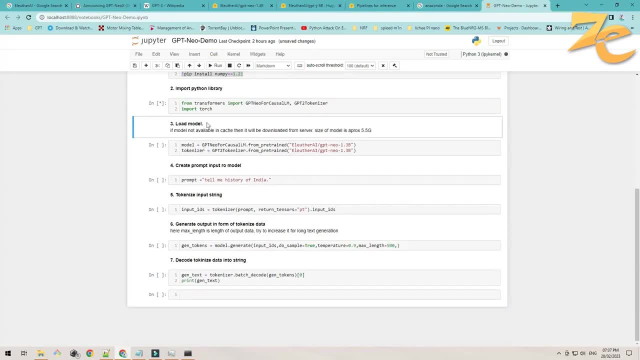 Here. Or. You. Can. Run. This. Command. This. Will. 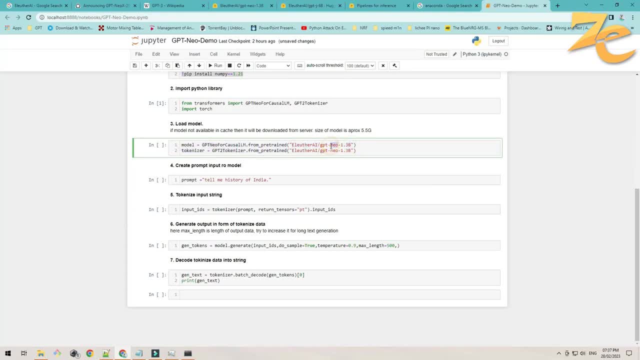 Include. The. Model. Which. Is. GPT. New. If. You. 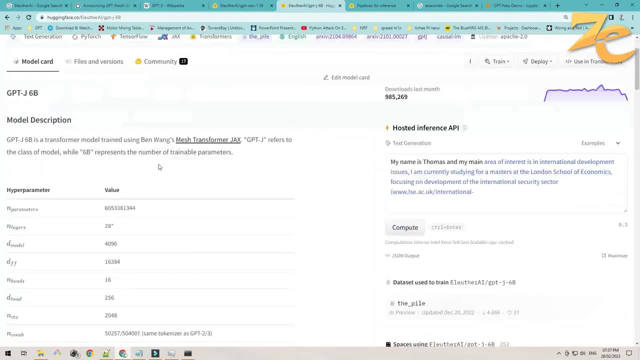 Want. Other. Model. You. Can. Simply. Go. To. Website. 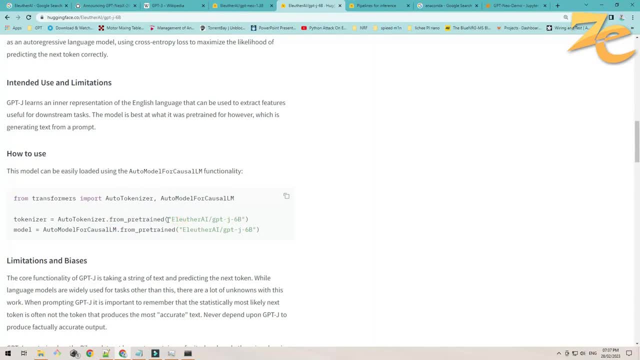 Here. Having. Paces. Are. The. Website. Which. Contain. All. 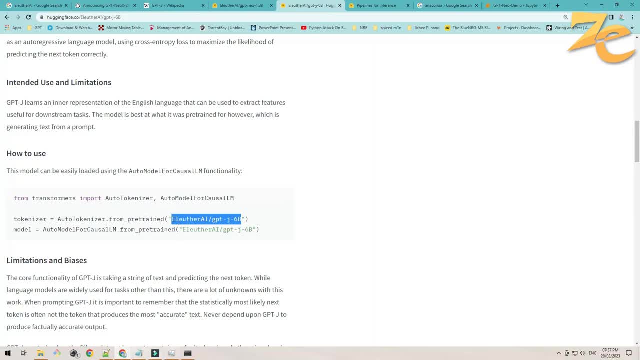 Of. The. This. For. Anaconda. So. You. Don't. Necessarily. 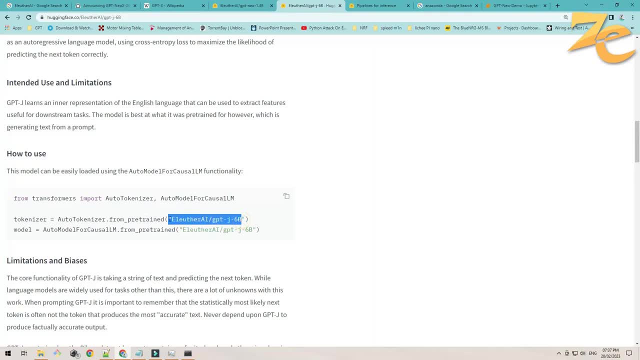 It. Will. Download. Always. It. Will. Only. Download. First. 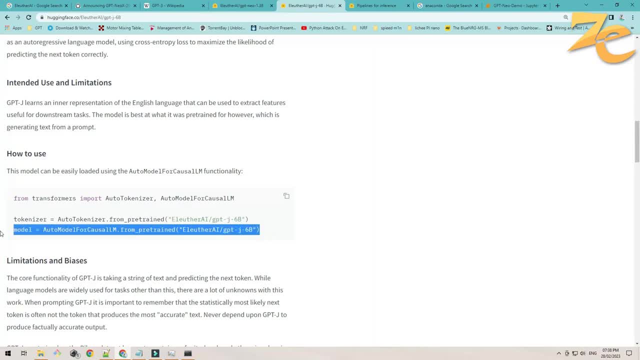 Time. But. This. Model. Is. Around. 24 GB. For. The. 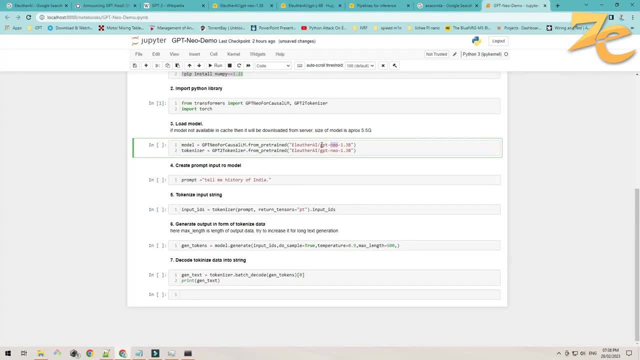 Float. 32. And. By. GPT. New. It. Is. Capable. 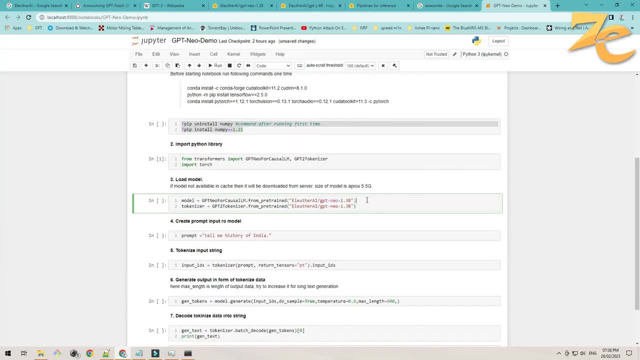 To. Run. On. My. Machine. So. I. Just. Already. 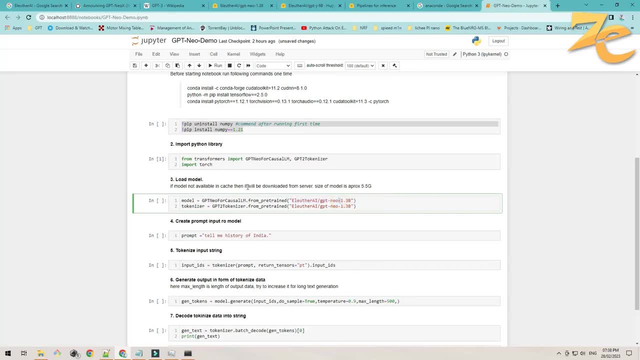 Have. Downloaded. It. Will. Take. Around. You. 5. To. 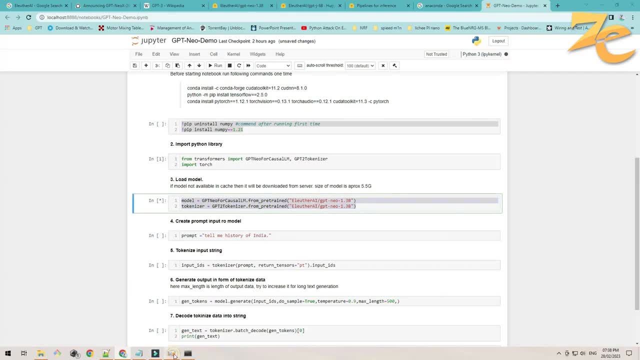 5. 1. Gig. Sub. Network. Bandwidth. It. Goes. Around. 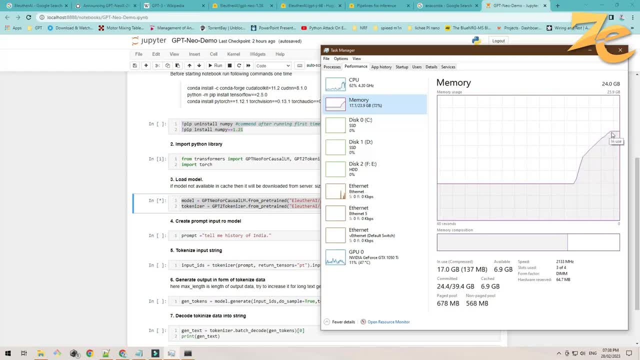 Here. Currently. It. Is. Available. So. It. Picks. Up. 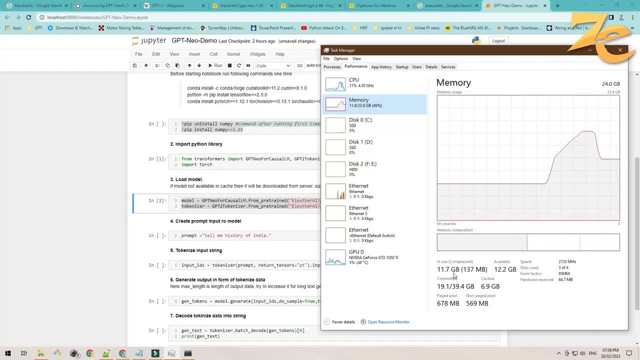 To. The. Like. 11. Or. 12. GB. And. It. 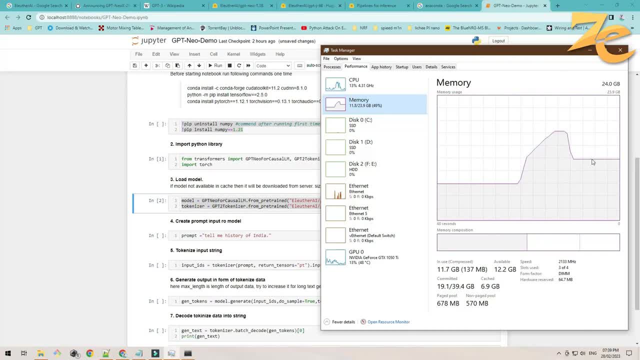 Is. Now. Running. On. Around. This. 6. Or. Something. 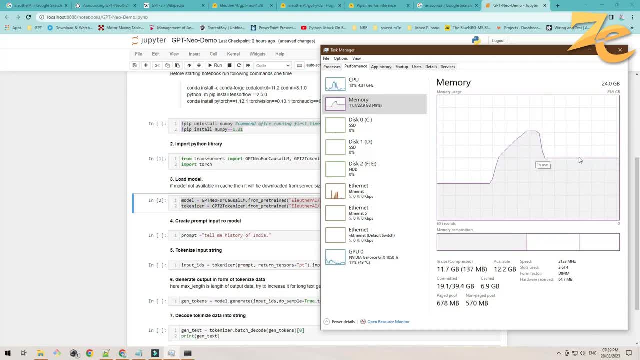 Loaded. Here. Successfully. And. Currently. It. Is. In. Memory. 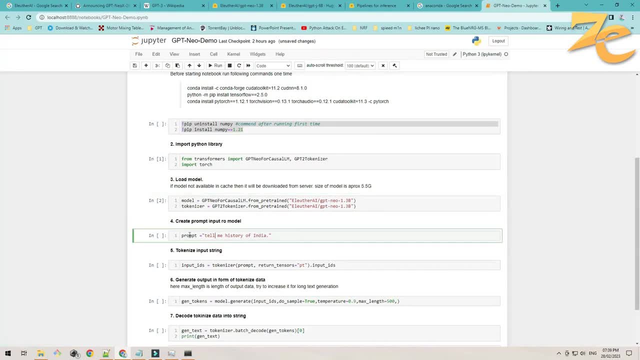 Now. We. Are. Not. Using. The. Model. That. Why. 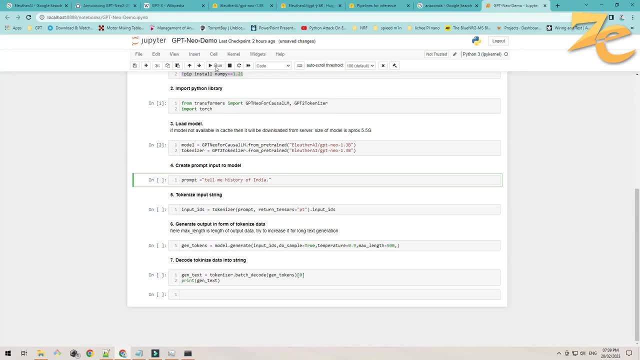 It. Is. Just. Constant. Okay. So. Our. Step. Is. 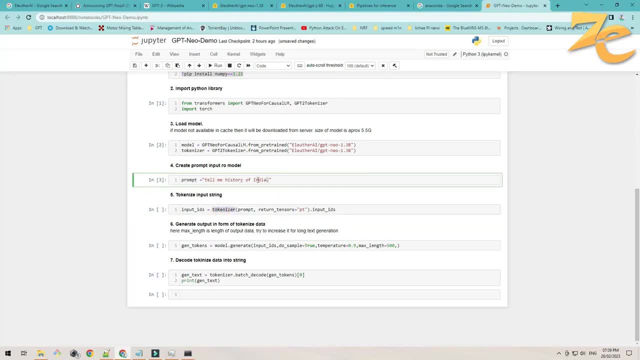 Completed. Let's. Look. At. The. Model. And. The. Symbols. 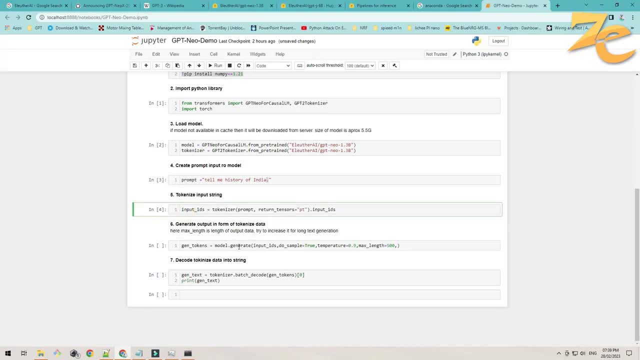 In. That. String. And. We. Get. The. Tokenized. String. 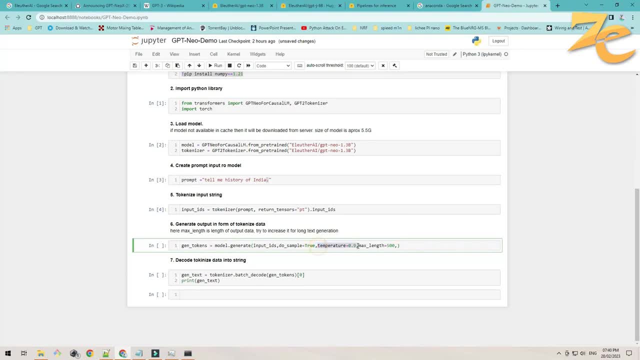 Now. We. Will. Pass. The. Tokenized. String. To. The. 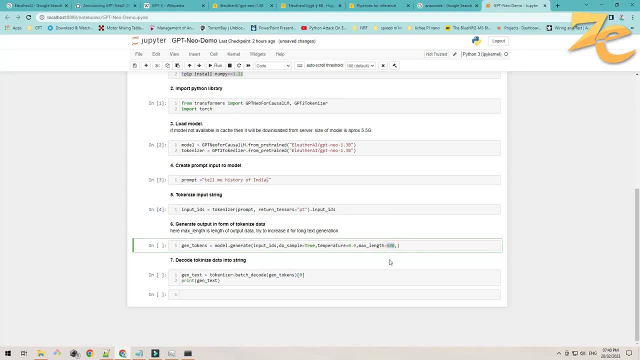 Model. Generator. Sorry. The. Tokenization. Will. Be. Taken. If.